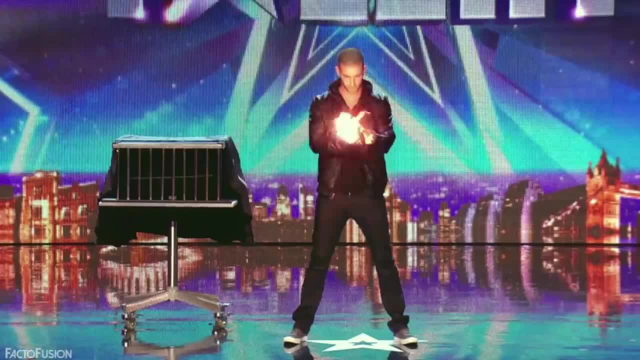 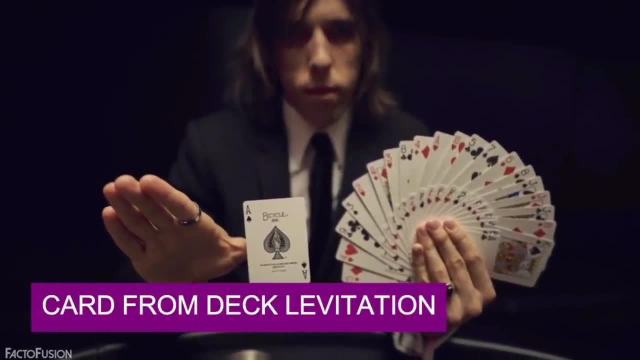 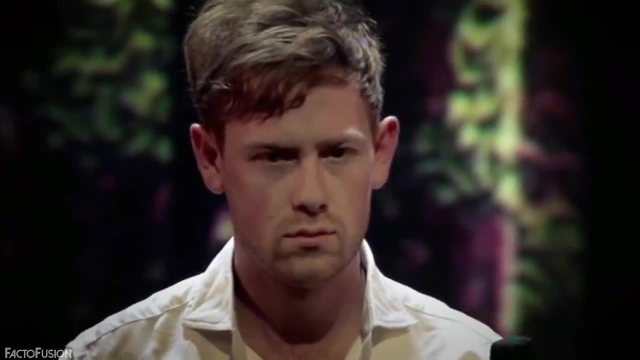 So there's actually no magic, just the quick momentum of time. I think you just missed that, isn't it? Card from Deck Levitation. It's almost impossible to know what the other person is thinking or watching, but not too hard for a magician. 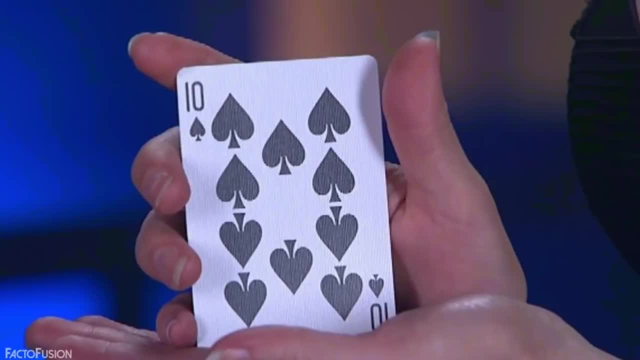 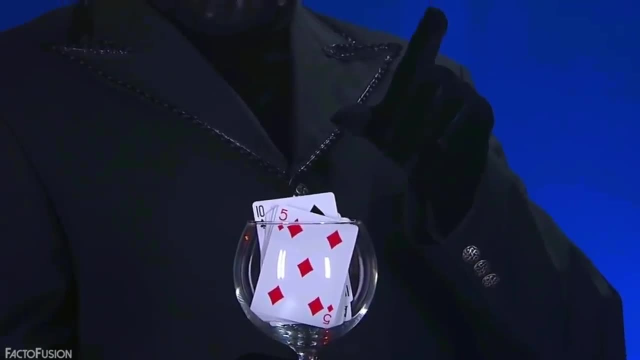 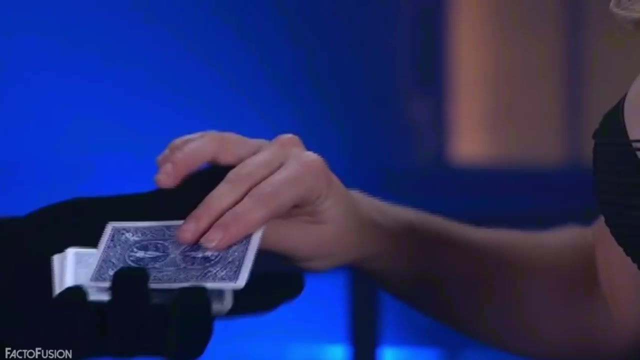 In this trick, the magician tells to choose any card at random from the deck and then places it back into the deck. He places the deck of card in a glass and does some magical gestures, and the card is popped out. The secret lies here: The card chosen at random is placed back into the deck where the magician wanted it to be. 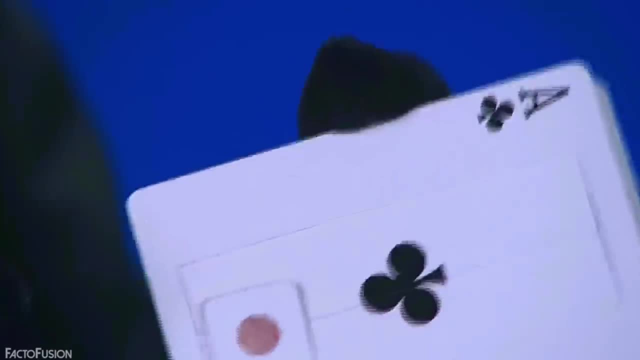 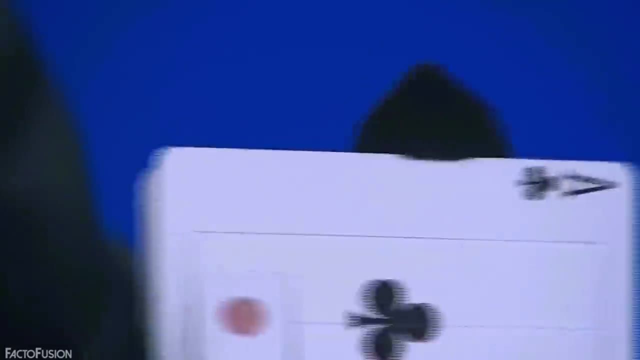 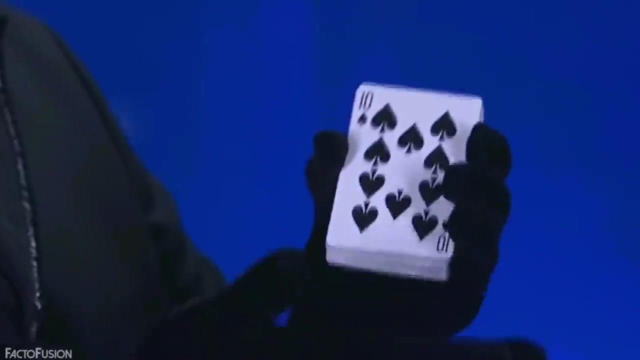 He places the remaining cards back over the deck, which is supported by a special card at the end. The special card is supported by a counterweight that moves a small pad upwards. when the card is turned upside down, The pad has a small dot of wax that sticks to the card and moves the card upwards, making it pop out of the deck. 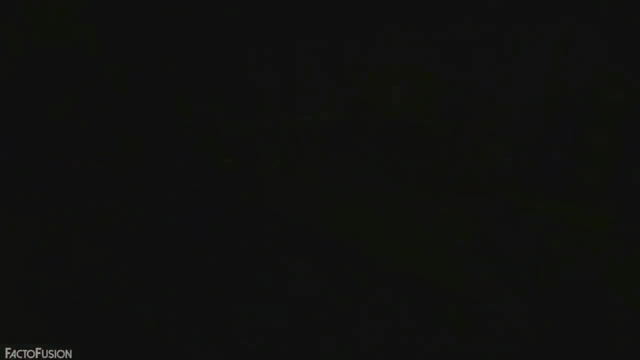 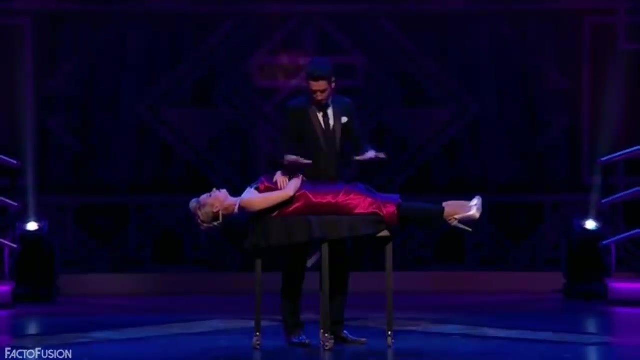 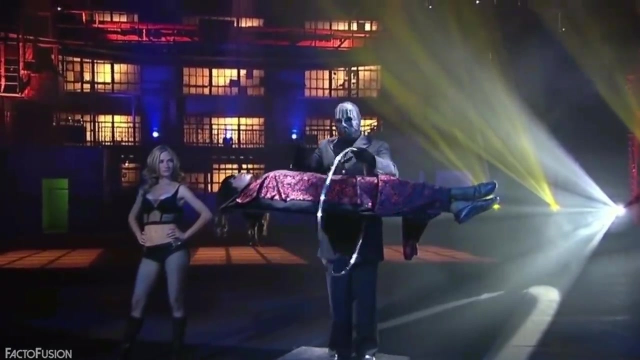 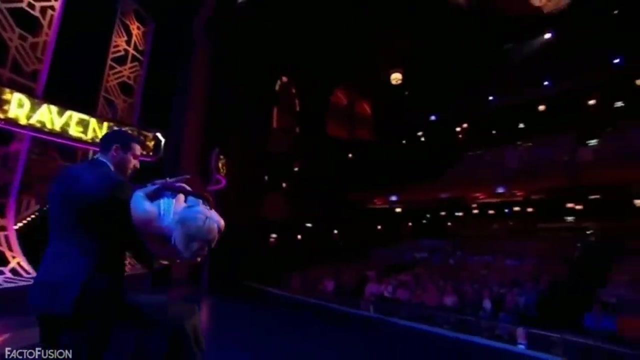 Girl Levitating in Air. We all must have seen a beautiful girl that is floating in the air on a plank of wood, And a ring is also passed around her neck To ensure the audience that it is not supported by strings or rods. Now that's really magic? No, not at all. 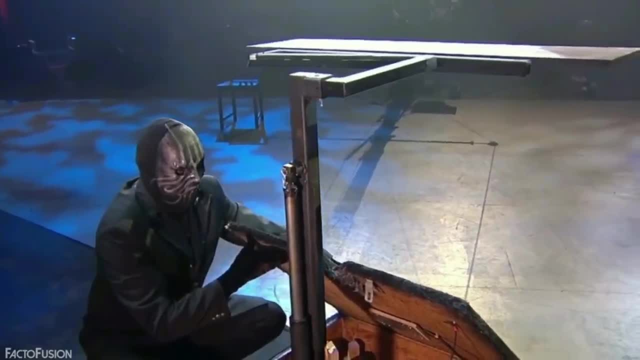 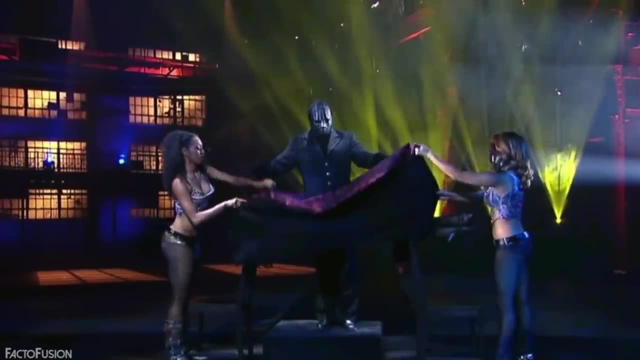 The plank of wood is supported by a strong hydraulic piston mechanism to hold the plank up in the air. The mechanism is hidden when the magician steps on the platform and takes his position. Under the foot of the magician, there is a button to control the motion of the plank. 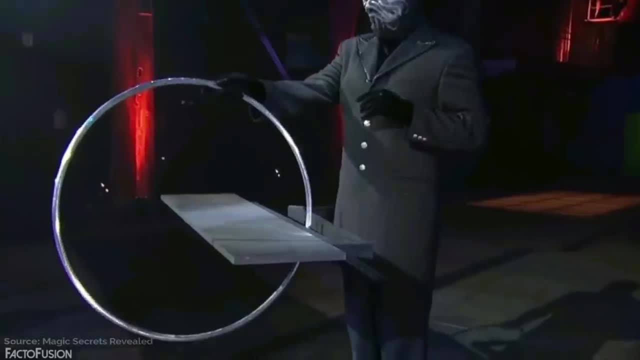 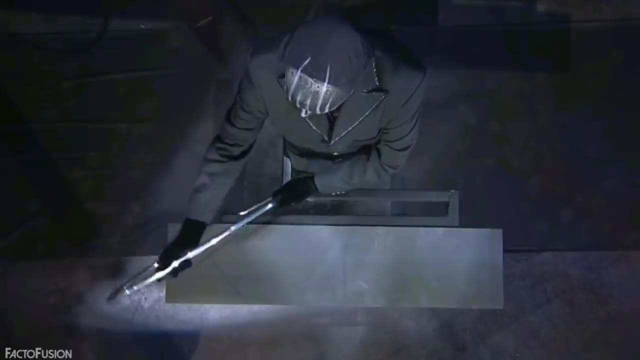 But how did it then move the ring around? Well, that's a good question, But the answer lies in the S-shaped design of the support rod. It can easily move the ring to the end and repeat back the movement to get the exit. 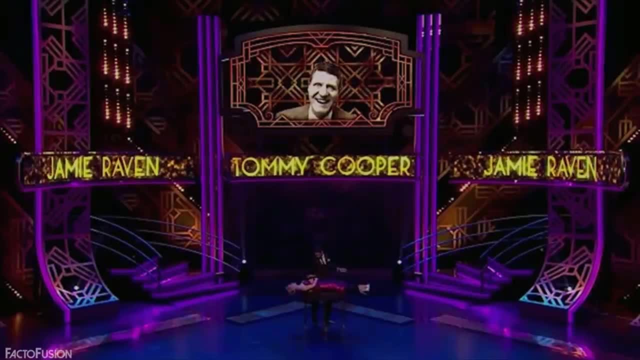 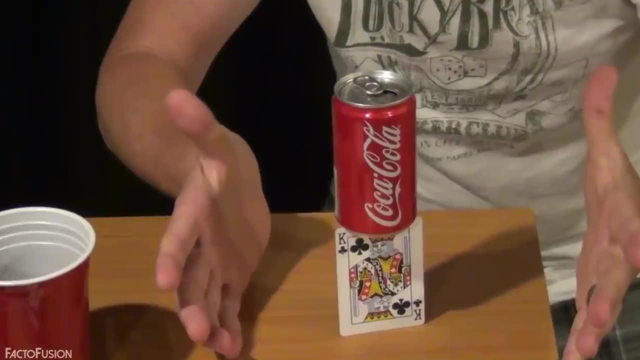 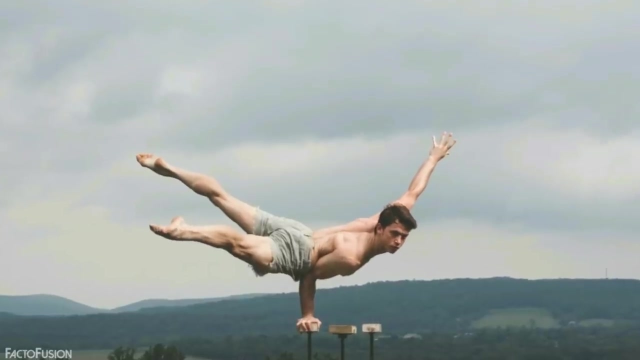 So there's no magic at all. It's just an illusion. Can on a Card. Making a bottle of can stand on a card is an incredible magic, But not when you know the secret behind it. We all have seen great balancing acts shown by magicians on the internet. 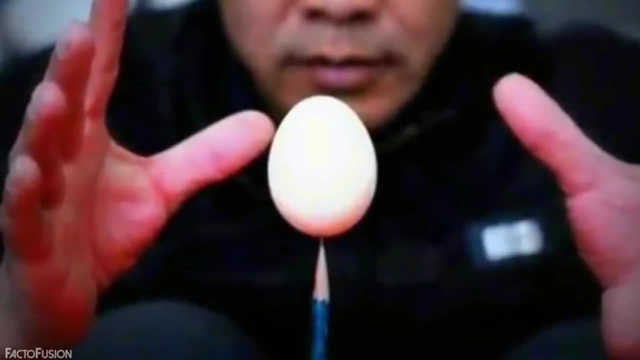 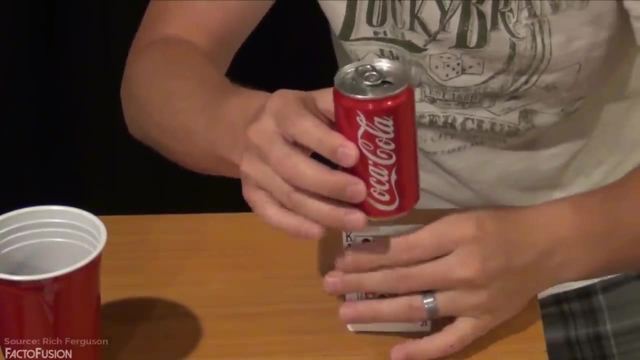 But this is a special one. Let's see how it's done. The magician takes a card and places a can on top of it, Then does some magical acts of insanity And there you have it: The can is standing on top of the card. 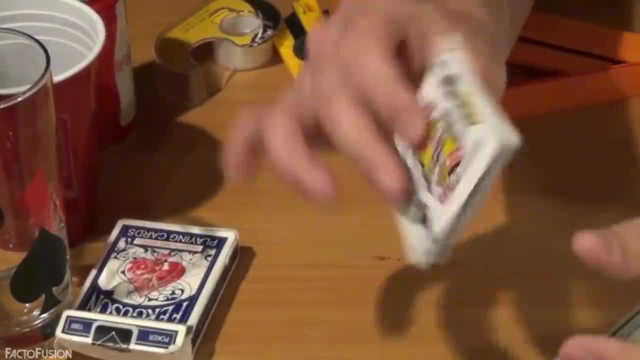 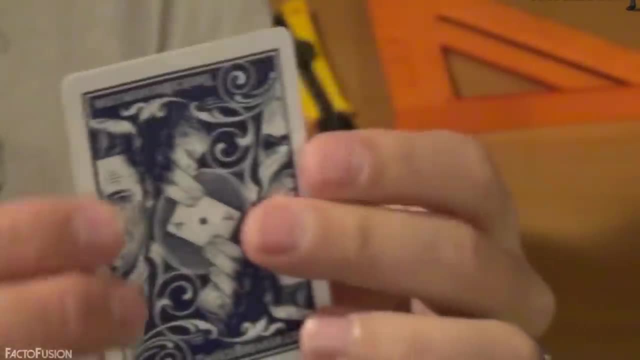 But when you take a look at the back of the card, it's actually two cards stuck together and folded from the center. that forms a T-shape. That's easy to make the can or a bottle stand over a card, But it's not easy. 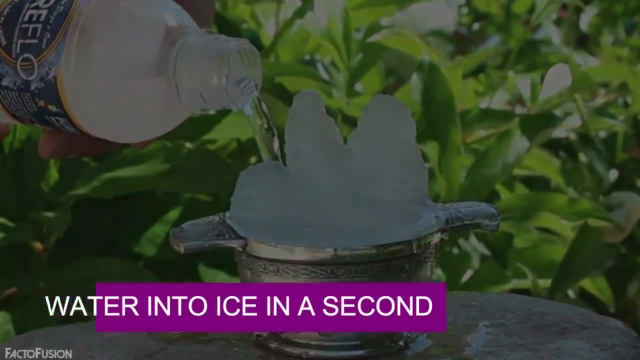 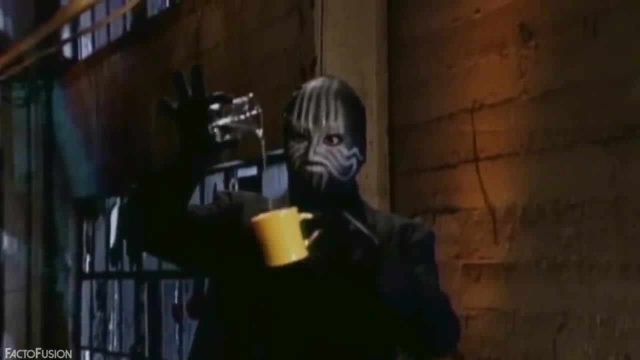 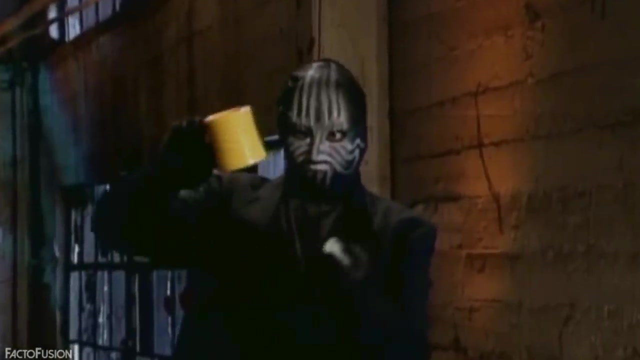 Water into ice in a second. Can you turn water into ice in a second, even with a deep freezer? No, But a magician can Watch this carefully. The magician pours water in a cup and instantly turns it into a piece of ice. How did he do it? Does he have a freezer in his hands? 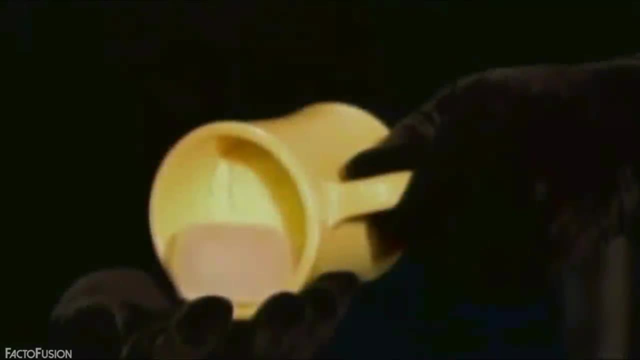 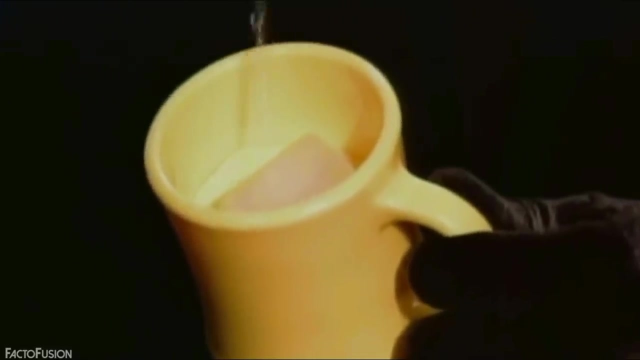 The cup already contained a piece of ice in it and a sponge of same color at the bottom of the cup. The water is absorbed by the sponge and what is left when the cup is turned upside down is the ice- the magic David Copperfield's Death Saw. 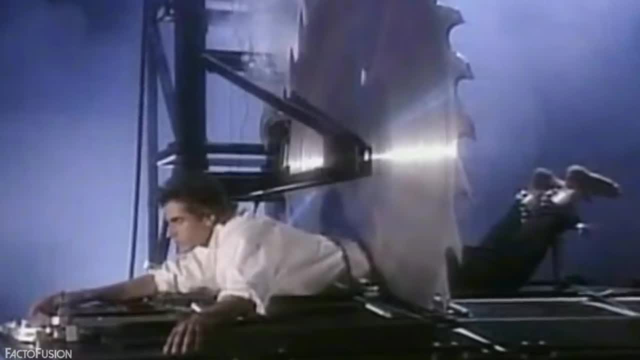 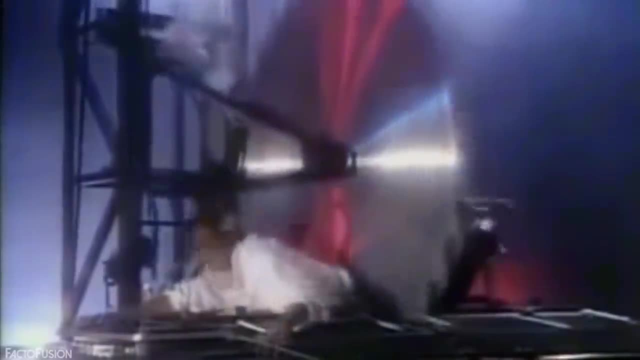 David Copperfield, the much-known classic time magician, performed the act of death saw magic, in which he split apart himself into two pieces using a giant saw blade. That was really a great piece of illusion created by him, But here's the actual secret behind it. 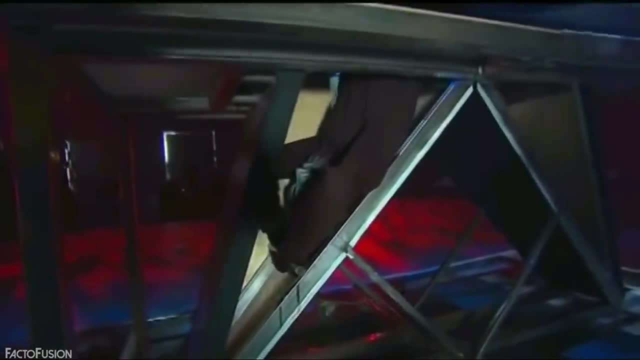 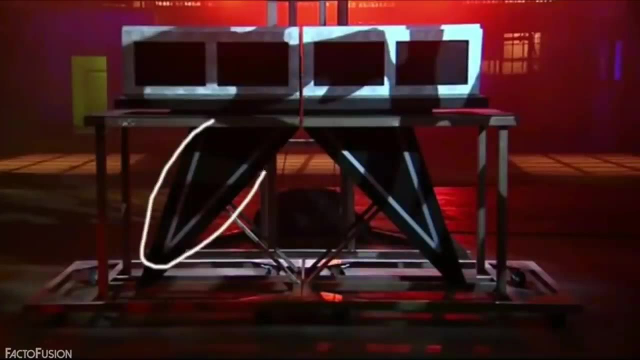 It's not just Copperfield in this act alone, but supported by one of his assistants for the later part of his body. The actual positioning is done in such a way that together they seem to be just as a single person. All the secret lies in the table beneath and the slight gap between the tables that can easily pass the saw blade from that. 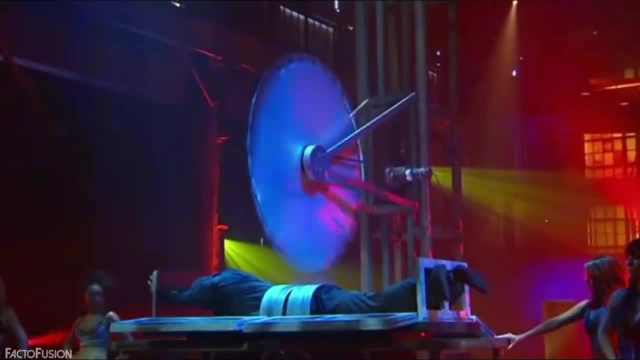 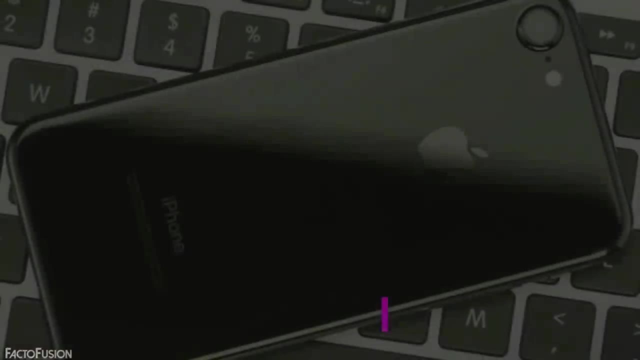 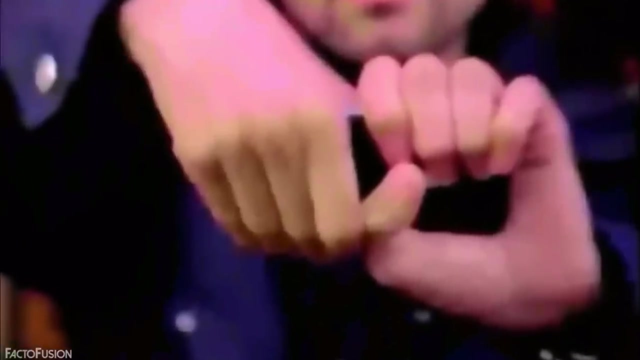 The body of Copperfield is bent into the table, while the assistant's upper body is hidden in the table below. But at the end, hats off to the great piece of illusion and synchronization created by Copperfield. Twisting an iPhone. Have you ever tried to twist your iPhone from its center? 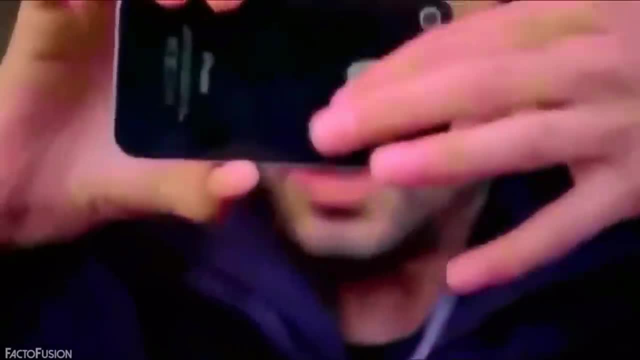 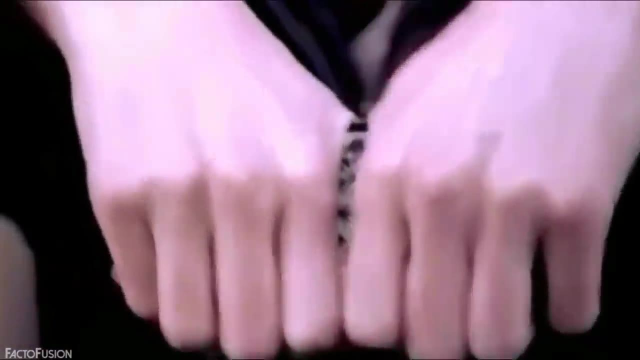 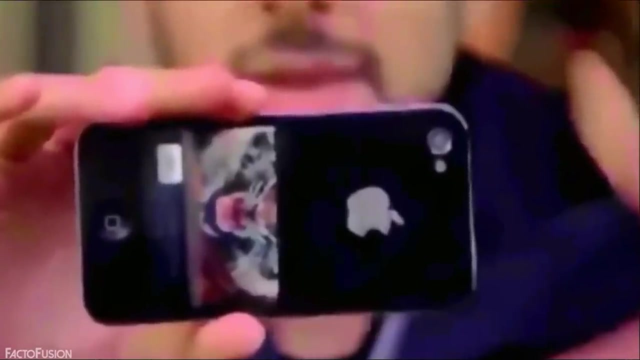 Obviously not, But Dynamo has done it in front of people on streets. He took an iPhone and magically twisted it from its center to half-screen and half-back position. That's insane. How did he do it? Well, here's the actual trick behind it. 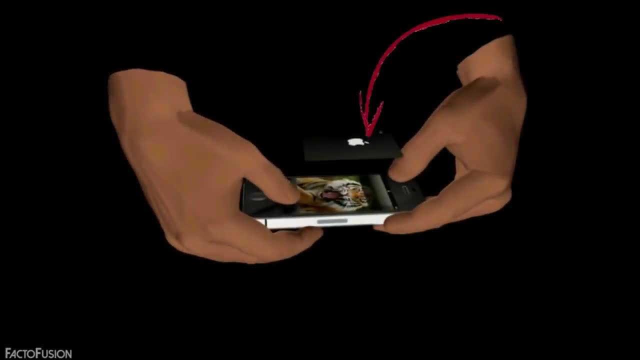 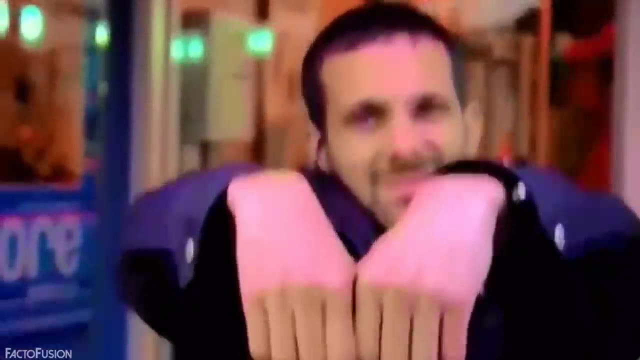 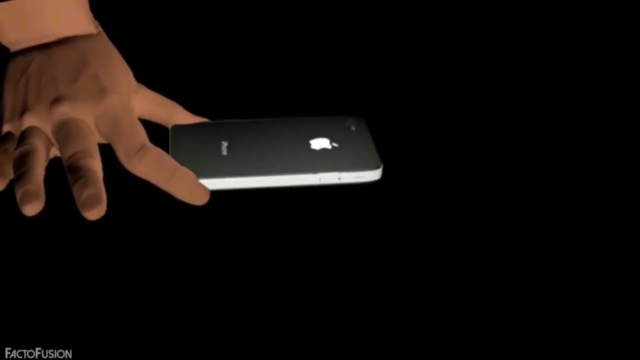 Dynamo took an exact half-back cover of iPhone and placed it carefully holding over the screen, Now showing the audience the back of iPhone. at first, He covered the iPhone with both of his hands and instead of twisting it, actually he just rotated the iPhone entirely to screen side, with a half-back cover placed over it. 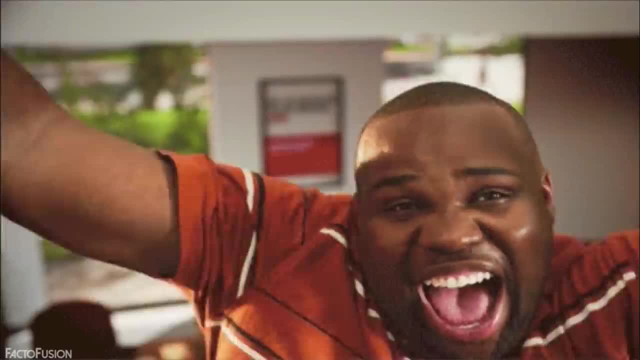 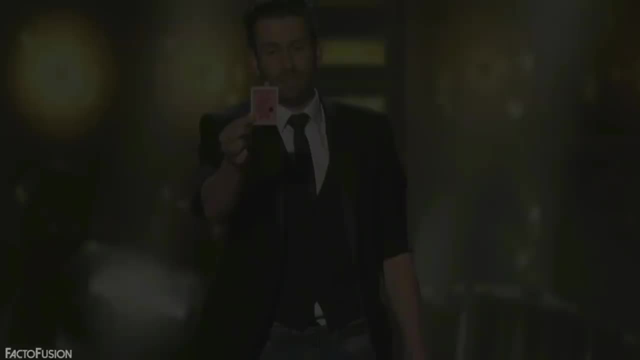 Go, try out this trick with your friends and make them scream like crazy. Jamie Ravan's Lemon Trick. Jamie Ravan, the magician, famous for his acts in Britain's Got Talent. In his final magic he got a signed note by Alicia out from the lemon. 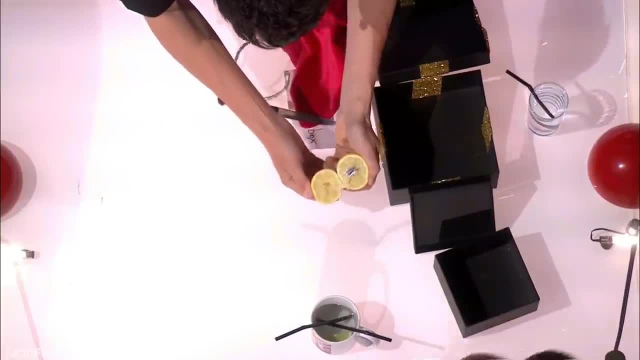 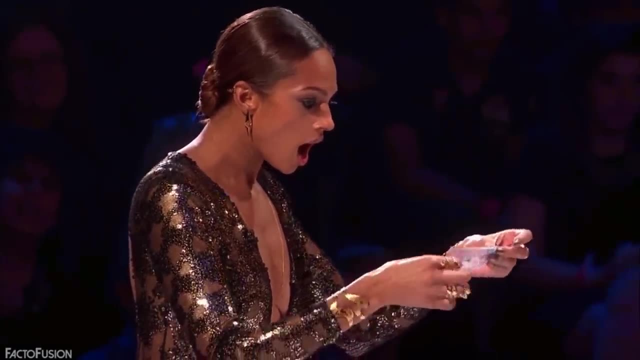 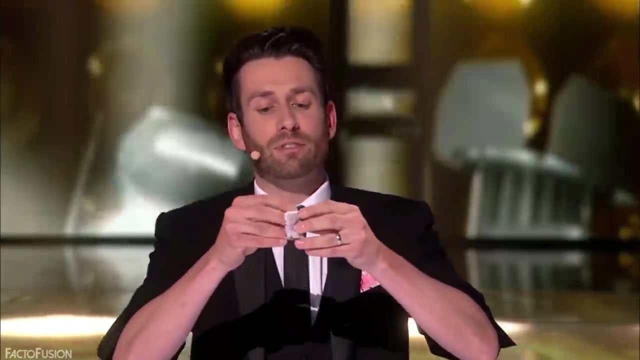 That was kept intact in front of her since the start of the show. Could you take out the note for me? You can't be kidding me. Does that have your name on it? Is that your name, If you take a closer look, while he was folding the note. 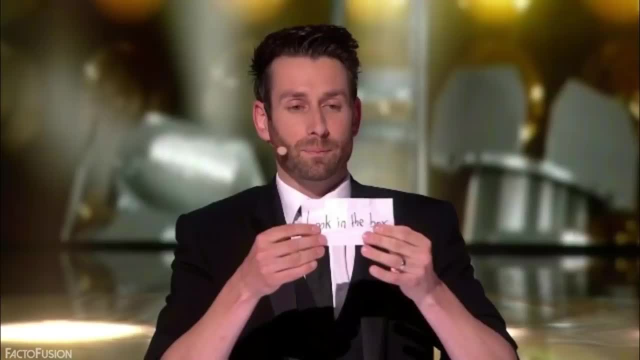 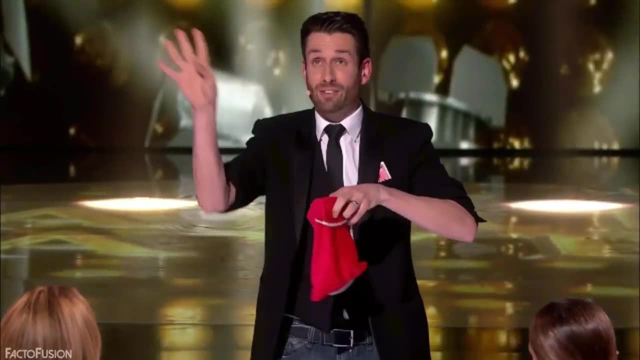 He had a palm piece of paper in his hand that he instantly switches to and shows the people. Now, with signed note still in his hand, he takes the bag from Alicia and drop the note into the bag very quickly And with an indication to the audience that there's nothing in his hands. 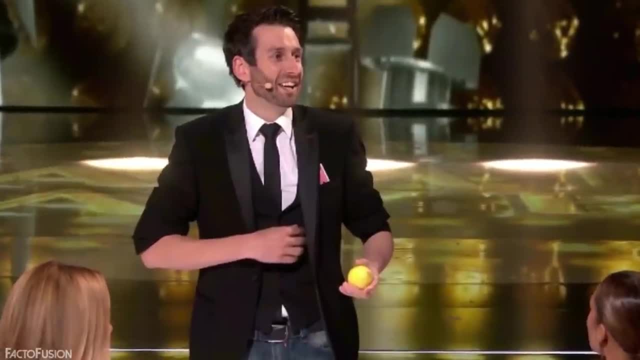 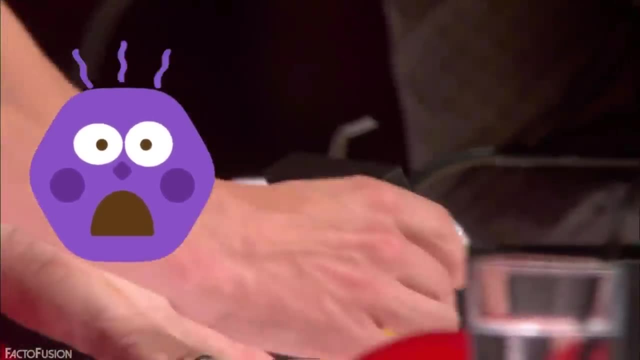 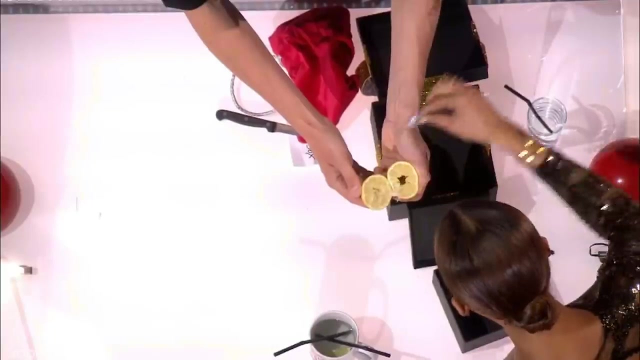 He reaches into the bag, stuffs the lemon with the note and takes it out very differently. He only shows one side of the lemon to the audience and cuts it very much differently. Have you ever tried to cut a lemon like that? Now, when Alicia took the note out of the lemon, he very quickly closes it and puts it away. 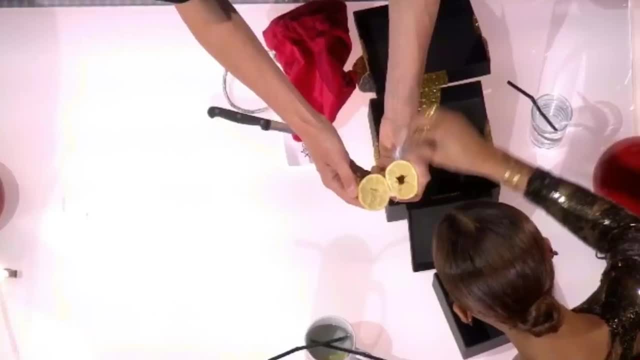 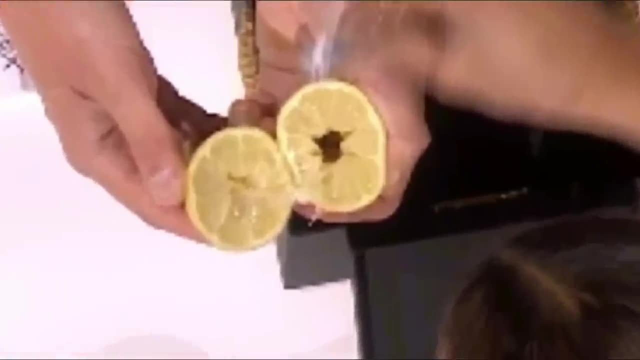 But let's take a closer look at it before. There's actually a hole in the lemon below, and that's clearly visible. It is this hole through which he stuffed the note inside the lemon and the magic was created. That's really great trick, Jemmy. 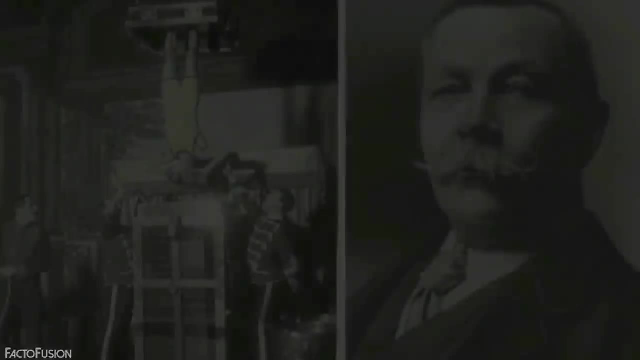 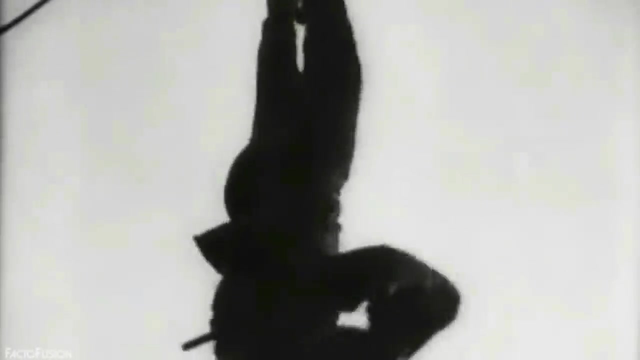 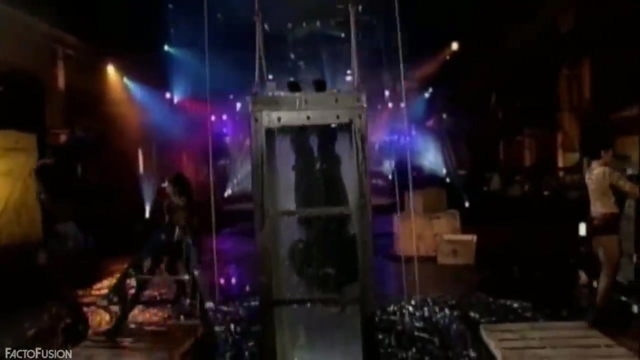 Houdini's Greatest Escape. The greatest and most sensational of all Houdini's escapes was, without a doubt, his Chinese water torture cell. In this trick, Houdini was to escape an extraordinary contraption resembling a fish tank. The tank is filled with water, while Houdini's players head down in full view of the audience. 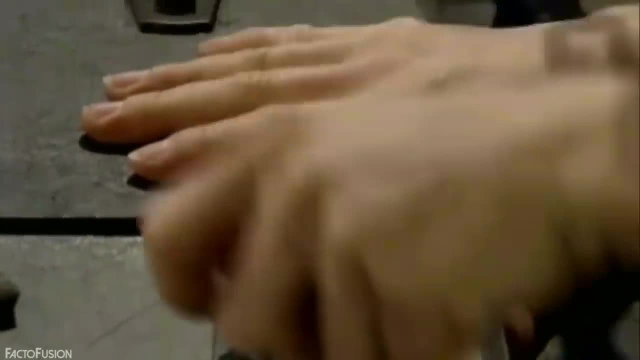 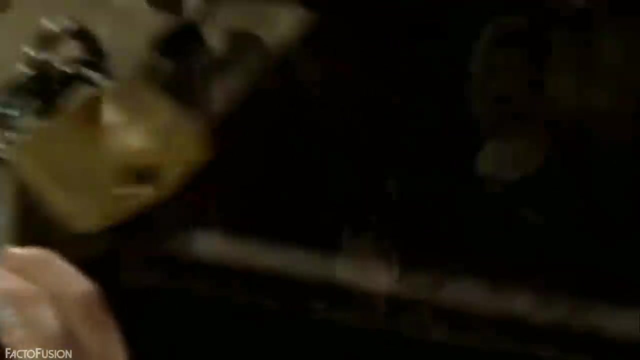 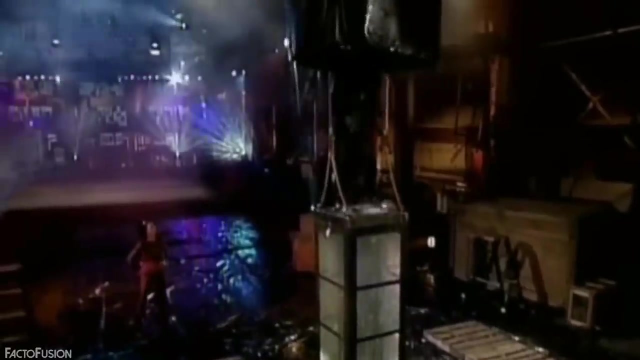 But how did he escape? in front of the audience, with all the contraptions on his body, The assistants lock Houdini upside down with genuine locks, but what we missed was they slide the pins out of the hinges holding the lock. Also, the handcuffs are specially designed to get open with just a little force and finally making the magician escape.